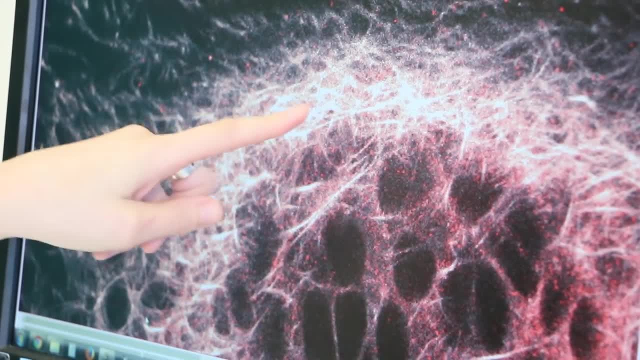 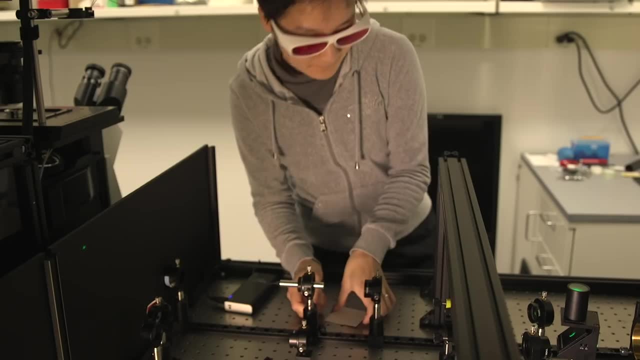 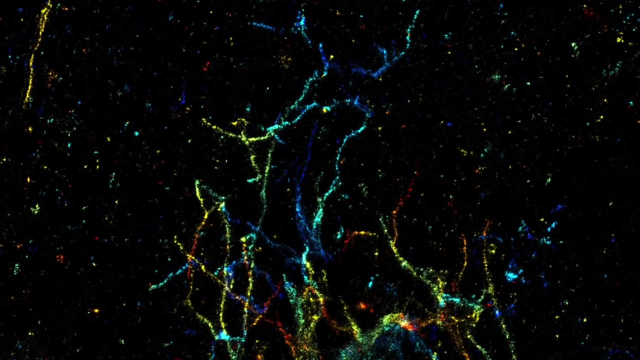 tissues lost or damaged from injury and disease. Medical Imaging faculty are developing advanced imaging for better ways to see into the body. You might build a super-resolution nanoscope that gives a more detailed view of the brain and help doctors see the progression of diseases like Alzheimer's. You'll be introduced to. 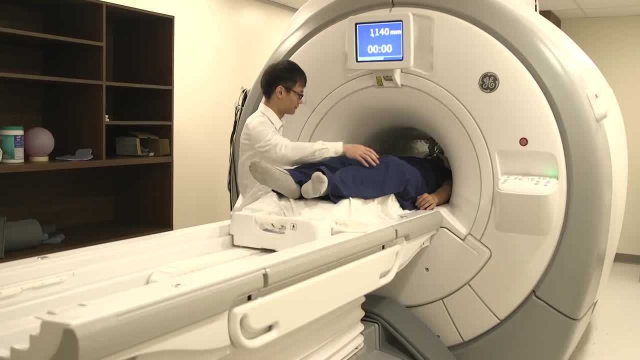 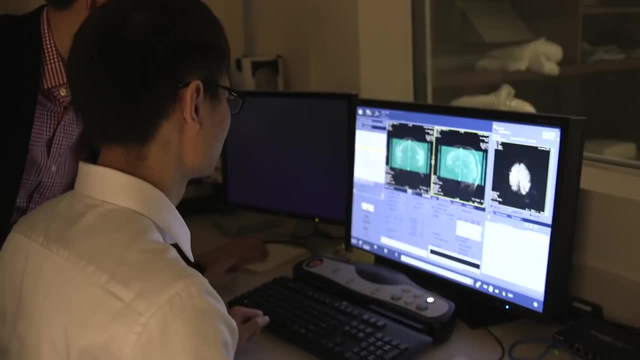 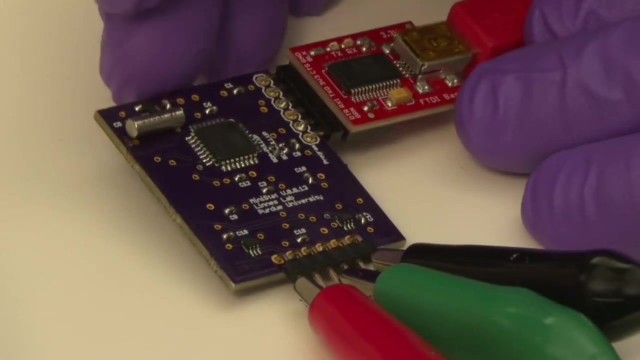 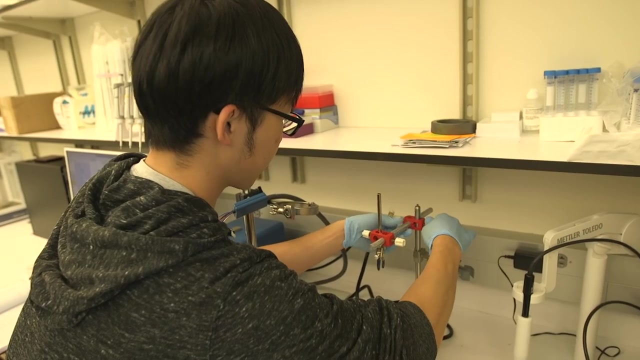 imaging tools, including ultrasound, advanced CT and functional MRI, and learn how improvements can help with diagnosis, characterization and treatment of diseases. Medical Instrumentation faculty address all aspects of instrumentation, design and application. You will learn about engineering new medical devices and optimizing existing devices. You'll learn the engineering science required. 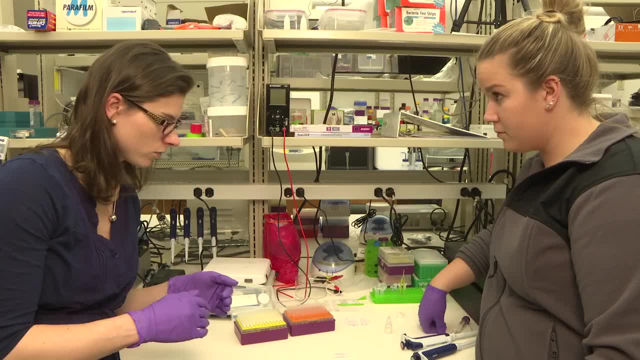 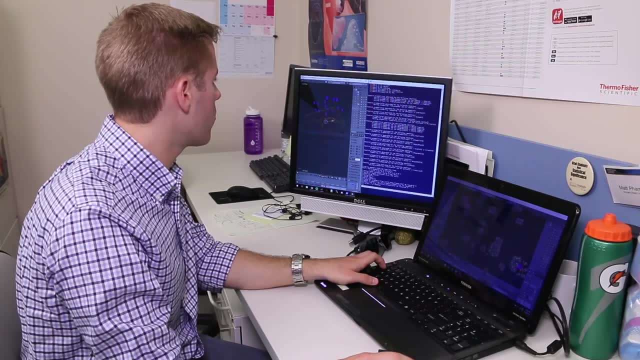 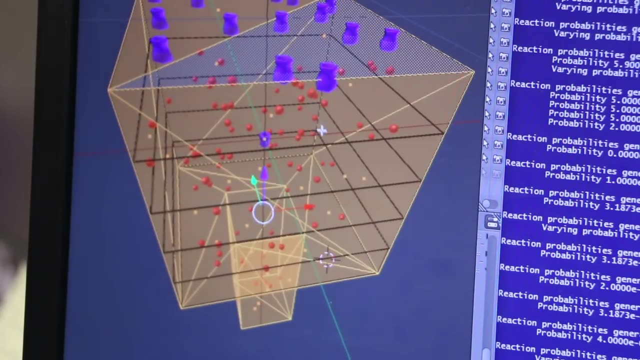 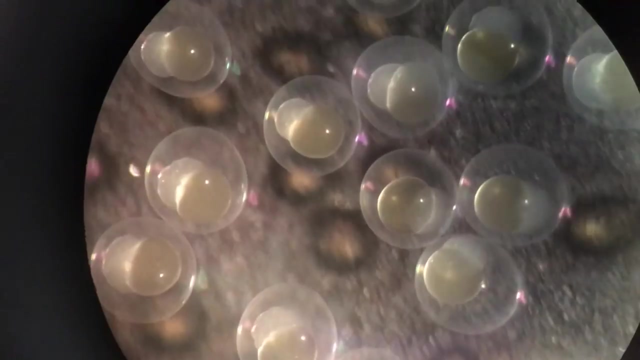 for testing and evaluating human physiology. You can also work developing cost-saving diagnostic tools for use in developing countries or remote areas, And quantitative cellular and systems engineering area. researchers work with mathematical modeling, systems analysis and engineering computation tools. You might study the role that proteins play in the growth and 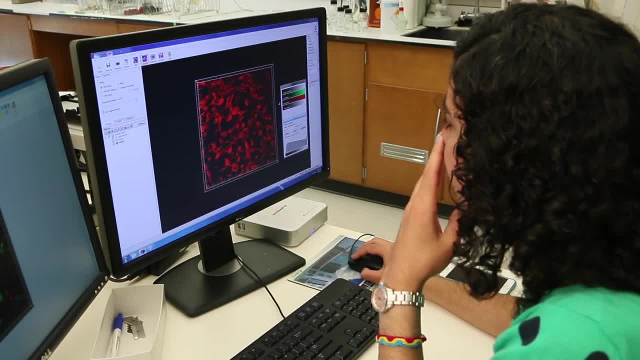 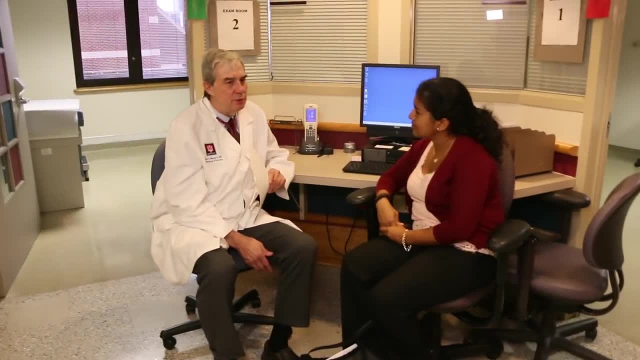 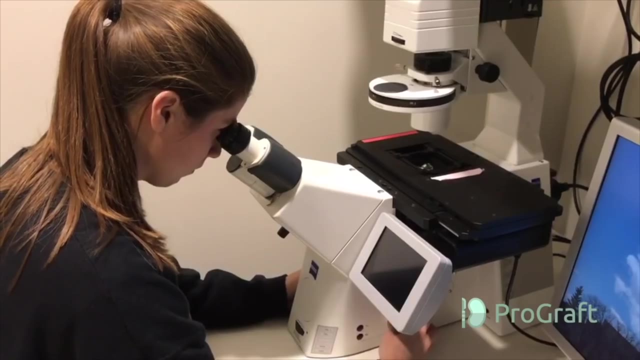 development of animals or make a discovery that helps researchers develop treatments to regrow tissues and organs in human patients. Your work could also help ensure that medical treatments in hospitals are provided in an efficient manner. Our undergraduate program is intentionally very hands-on. Each semester, through senior design, our students take lab courses that are 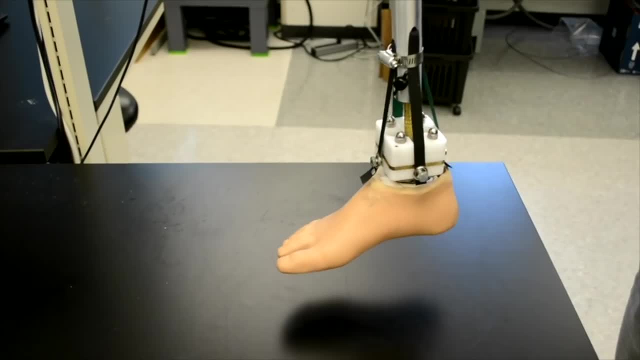 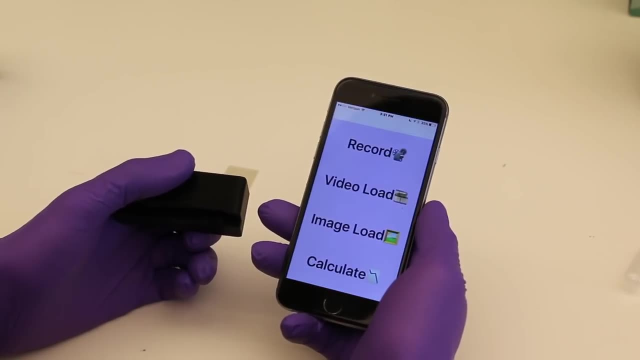 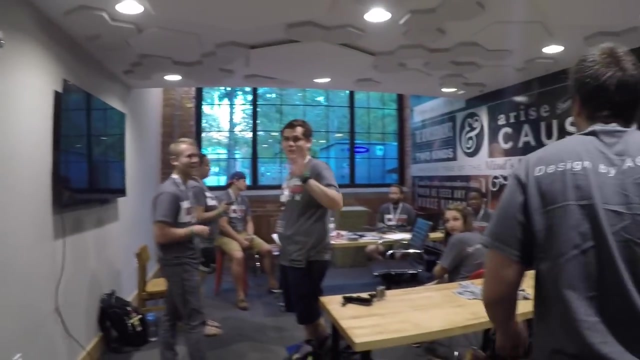 thematically linked to concurrent lecture classes, and then upper-level technical electives are used to specialize in your interest area. within biomedical engineering, which many students refer to as BME, Most BME students also take advantage of extracurriculars such as co-ops or 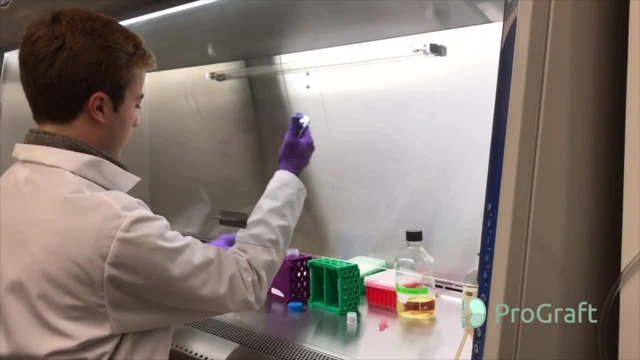 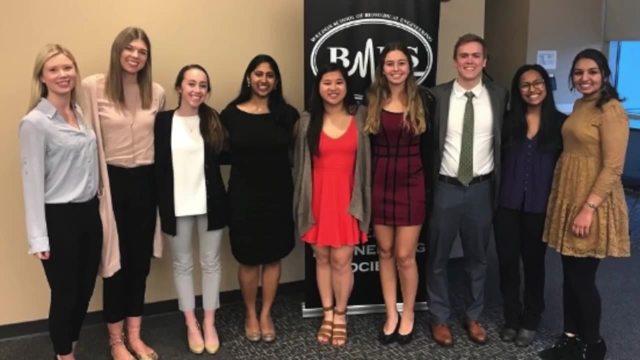 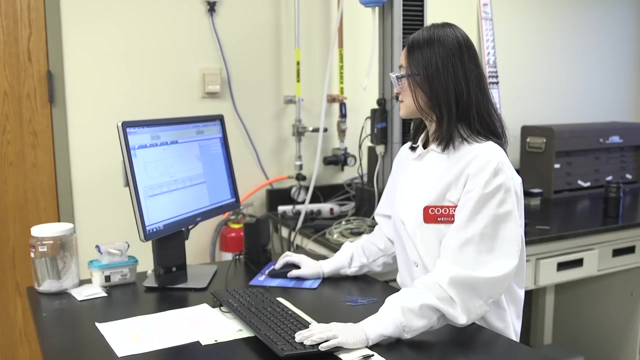 internships, undergraduate research in a professor's lab, clinical exposure opportunities, epics, study abroad and student organizations to help prepare themselves for life. after the bachelor's degree, Over half of our graduates go directly into industry, mostly in medical devices, But BME students are also hired by companies like Apple.